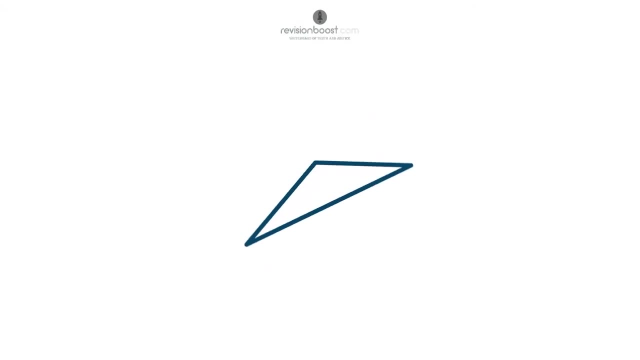 Rotations are the second type of transformation that we need to know about. When it comes to mathematically describing a rotation, there are three very important pieces of information that we need to give. First of all, we need to state the size of the rotation. 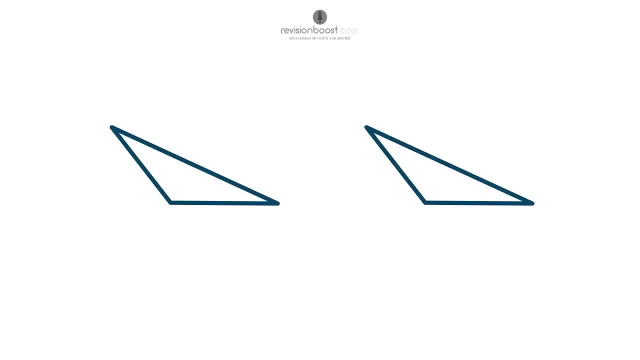 by using an angle. It's probably quite obvious that a 270 degree rotation is very different to a 30 degree rotation. Secondly, we also need to state the direction of the rotation. There are two possible options here. A clockwise rotation is a rotation that follows the same. 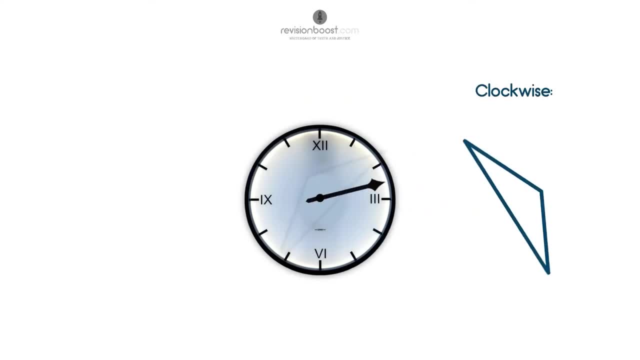 direction as the hands of a clock, whereas an anti-clockwise rotation is opposite to this. Finally, the third piece of information that we need to give when describing a rotation is the centre of rotation. So far, all of the rotations that we've looked at have been around. 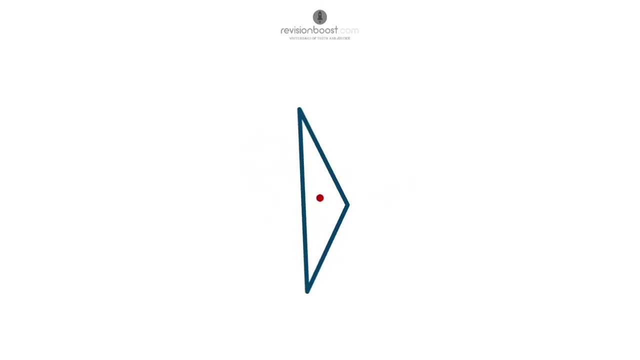 this point, which just so happens to be the middle of the triangle, But you can also use the triangle to describe the centre of the rotation. You can also use the triangle to describe the centre of the rotation. But you can also use the triangle to describe the centre of the rotation. 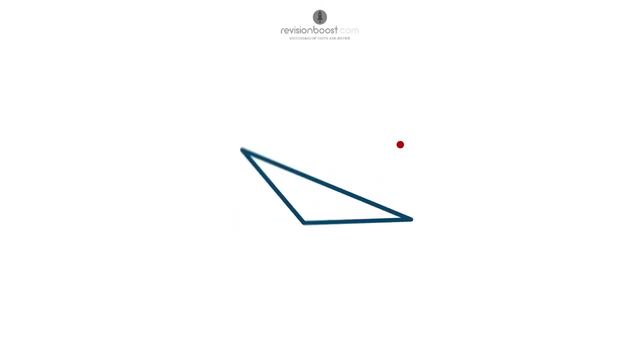 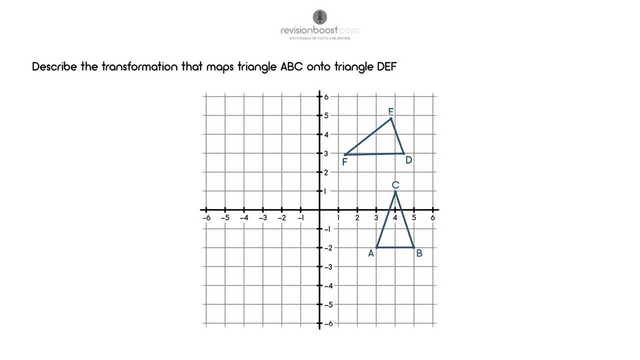 can also rotate around any other point, like this one, for example, or this one. So let's now imagine that we were given this diagram and again we were asked to describe the transformation that maps triangle ABC onto triangle DEF. Clearly, we can see that this is going to be a rotation of some sort. 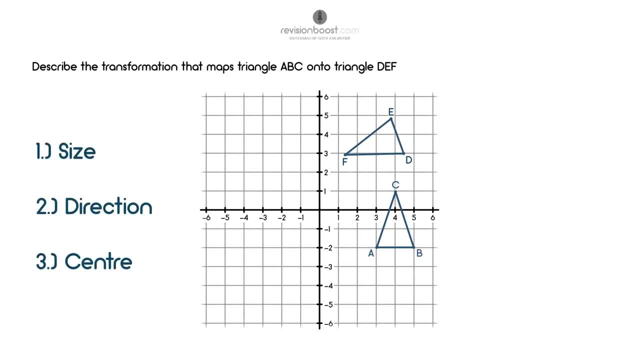 but how do we find these three important bits of information? Well, the first step is to find the center of rotation. This seems really tricky, but I'll show you a neat little hack for finding the center of rotation. First of all, you should pick a pair of corresponding vertices on both shapes. 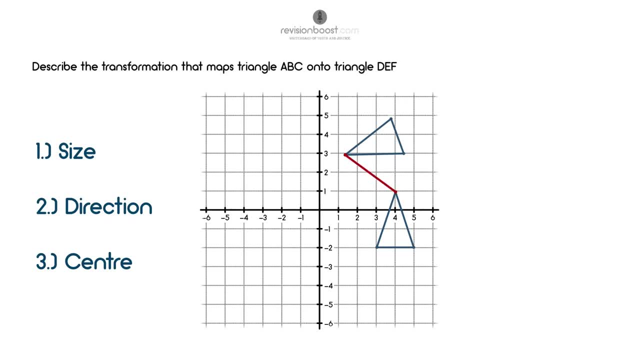 and connect them together with a line. It doesn't matter which pair you pick, so for this example, I'll randomly just choose this pair here. After connecting two corresponding points with a line, the next step is to draw the perpendicular bisector of this line. 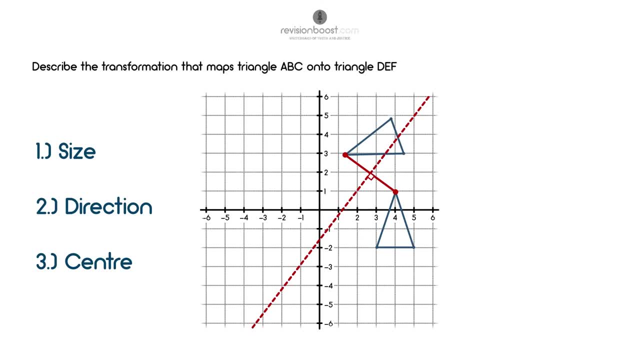 If you cast your mind back to our lesson on circle theorems, you'll remember that a perpendicular bisector is just a line that passes through the midpoint of another line at a right angle. So I'll mark on the midpoint like this, and then I'll use a protractor to draw an angle of 90 degrees. 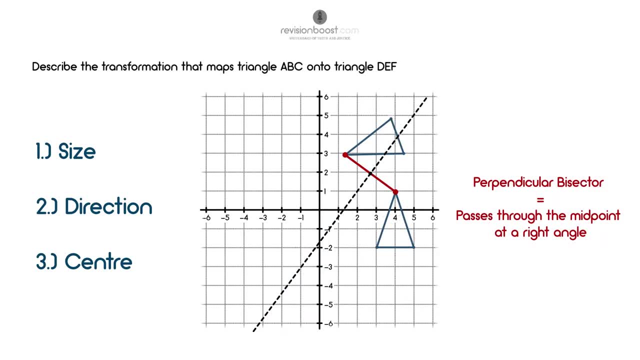 which means that this here is the perpendicular bisector. Next, we need to repeat this process using a different pair of corresponding points. Again, it doesn't matter which pair we pick, so I'll leave these two here. First, I'll connect them with a line and then again I'll draw the perpendicular. 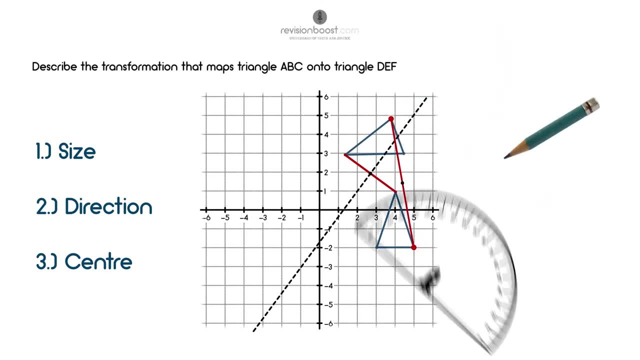 bisector of this line. Now, it just so happens to be the case that the center of rotation is the point at which these two perpendicular bisectors cross each other. If we change the size of this rotation slightly, you can see that this is true. The perpendicular bisectors always cross at this. 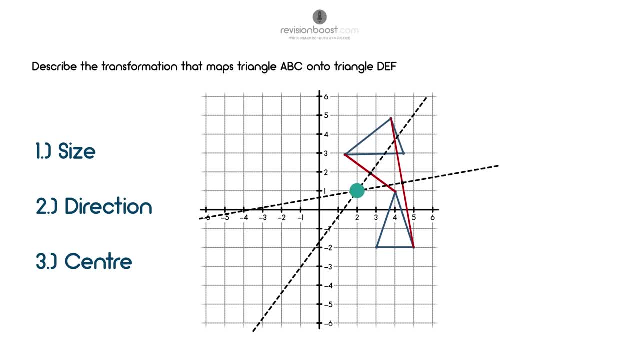 point. so we know that this is the center of rotation Two one. So this is great. now let's see if we can find the size of this rotation, Because we already know the center of rotation. finding the size is actually fairly simple. Imagine a clock face positioned at the 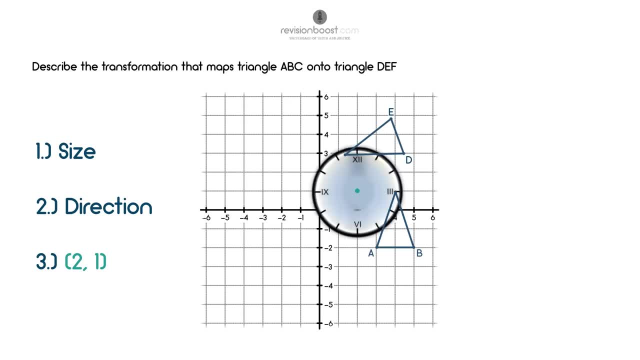 center of rotation, which we've already found, is this point here. two: one: Now imagine that we have a hand on this clock pointing to one of the vertices of triangle ABC. We can get to triangle DEF slightly Now. first of all, we can see that this is going to be an anti-clockwise rotation because 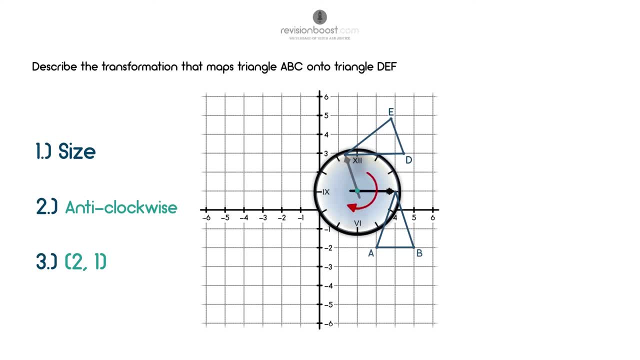 clocks normally spin around in this direction and we're going opposite to this. So now we know the center of rotation and we know the direction, but what about the size? Well, we can figure this out by using a ruler to mark the start and the end point of this clock hand, And then we just need 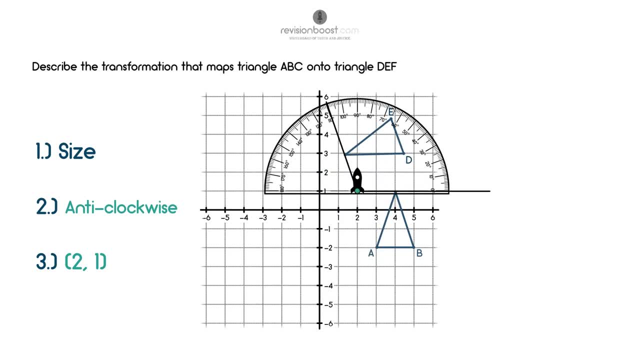 to use a protractor to measure the angle between these two lines. So in this case you can see that the transformation that maps triangle ABC onto triangle DEF is an anti-clockwise rotation of 110 degrees about the point two one Perfect. Remember these three bits of information when you're. 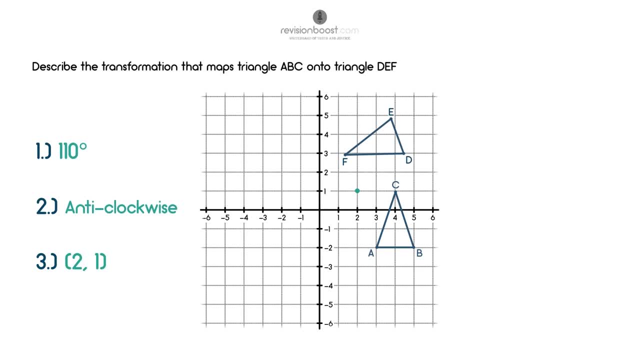 describing rotations, because they're all vitally important: The center of rotation, the size of rotation and the direction of the rotation.